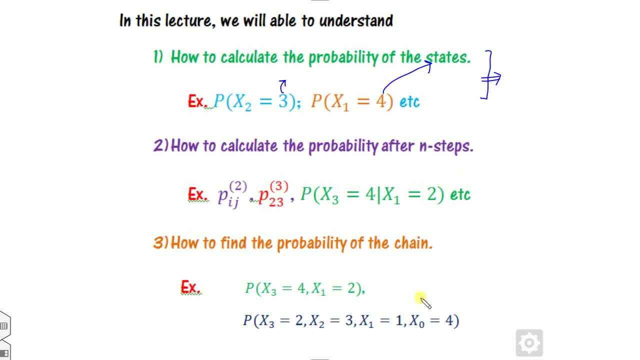 understand firstly the type one. similarly, in order to understand this, there is a need to understand the first and second board. so i just cover the type one here in order to understand it. so what we have studied in the lecture number one, that is, the transition probability matrix. 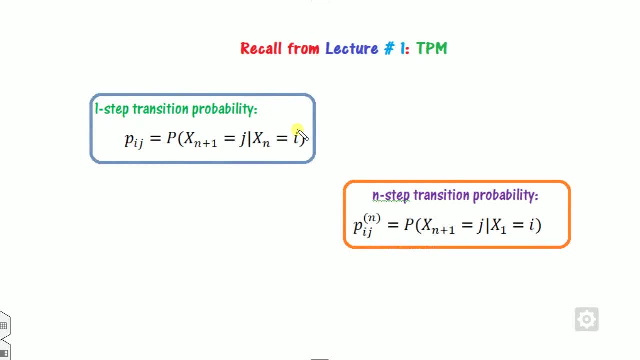 we have to return this first step. probability, that is, we have going from i to j, so that's why i j. what is the difference between the n plus 1 to n? that is a 1, so here is a 1.. look at for the. 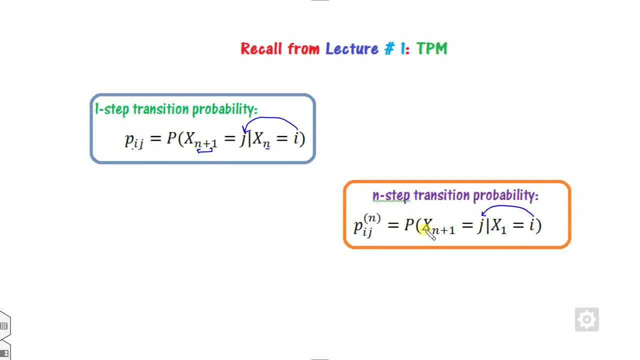 end step. you go from 1 to j, i to j, so that's why this is written as pi j. and what's the? the difference between the time period is n, so remember that always this is i, j and something is written. this is called as the time period, this is called as from where you start and this: 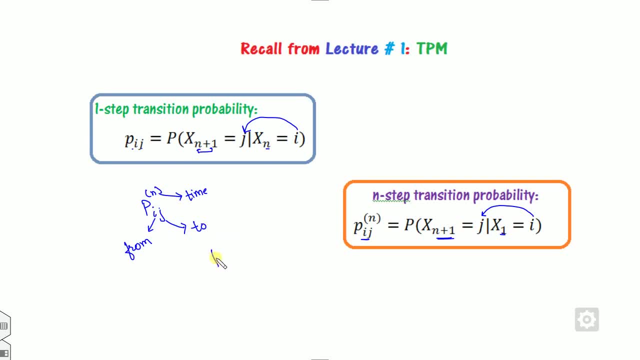 represent as where. to end that if i represent as p 2, 3 and represent as a 4, it means you start from the 2, reach at the stage third, after the four steps be like: this is the one step, this is the two step, this is the third step and this is the fourth step. so in this presentation i have explained. 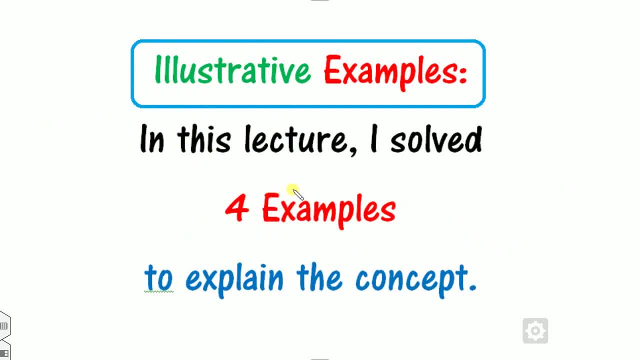 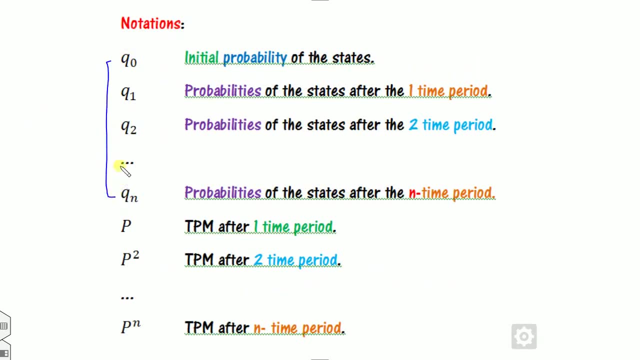 the four examples to solve to explain the concept. i can assure you that if you listen and solve these four examples very carefully, you will never fail in this markov chain example circuit. so as simply notations are there, first notation is representation of q. wherever i just represent a q, that is called 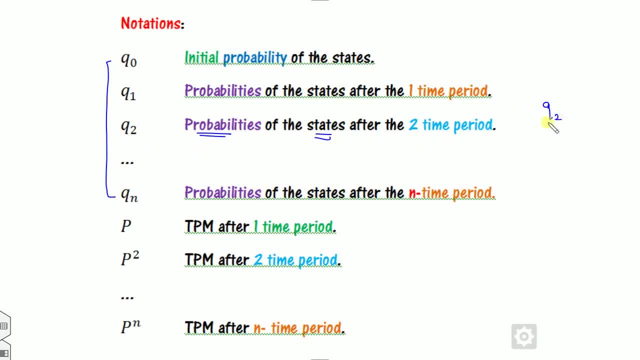 as the probability of the state. if i say q 2, it means the probability after the time 2. if i say q 4- probability after the time 4. q 0- 0 means the initial, so that's called as the initial probability. and wherever i represent the capital p, that is called as the tpm and the power represents that. 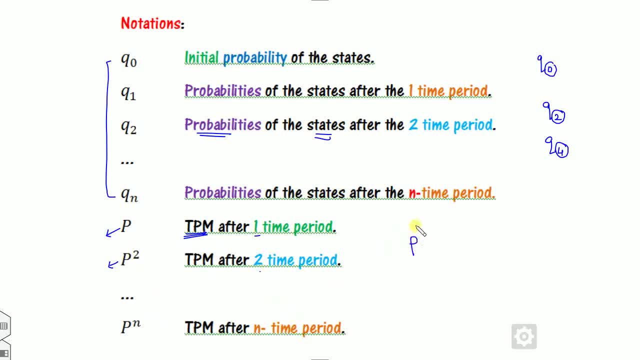 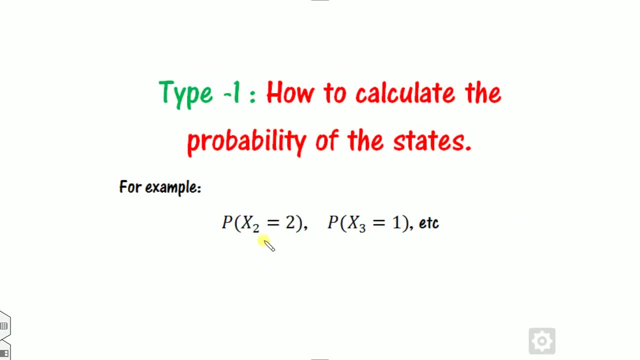 it's a one time, two time and three time and so on. so if i call p 4, this is called as the transition probability matrix after the four time periods. so how to solve the problems of the probability of the state. so look at that i am trying to solve. 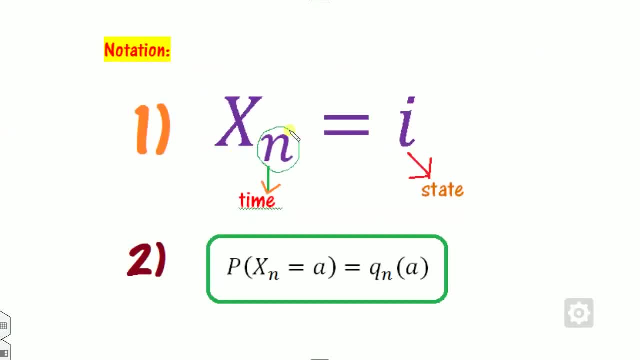 such type of the problems only. so, first of all, what is the notation that? so, whenever i just represent here, look at that x, 2 is equal to 2. so whatever we have written on the right hand side, this is called as the state, and whatever we have written the subscript is called. 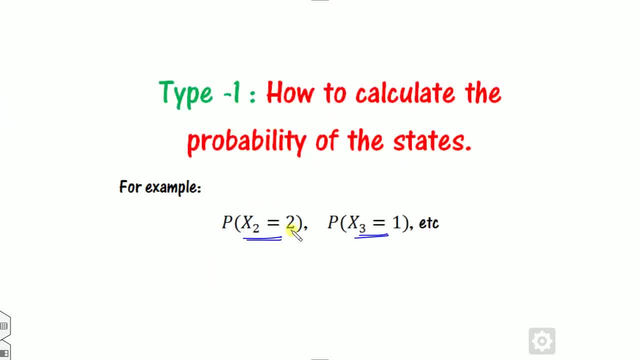 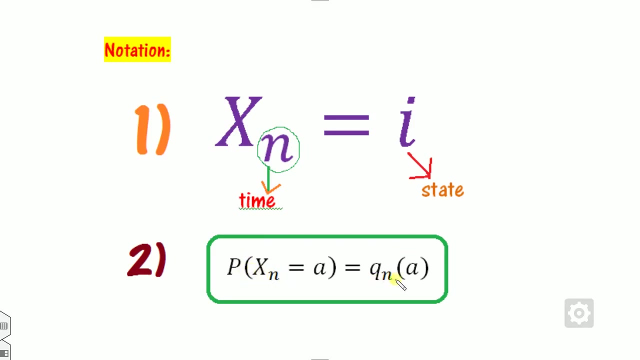 as the time. okay, so what is the meaning of it is? we have to reach at this stage, two after the time period two, we have to reach, we have to find the probability of the one after the time period three- and i use this notation whenever we have right here we call as q is the probability, this n always be here. 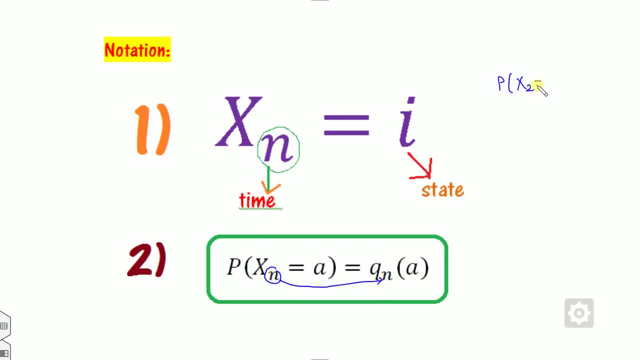 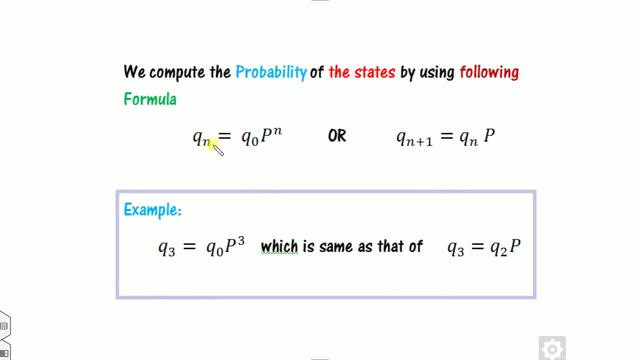 okay. so, for example, if i just want to calculate here, so it means i need to calculate the q 2, and after that we will check what is the answer at the fourth position. so let's start with them, and since here we need the q, so the formula for the q is this: 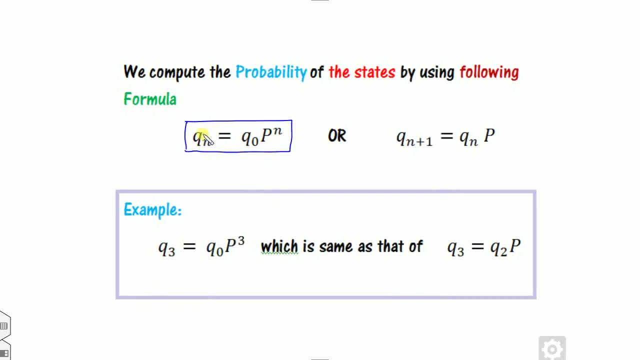 one. so how to remember them? qn, if i write qn is q0. so what is that? what is the difference between? the time length is n minus 0 is n, so i can write as n. on the other hand, you can also use like this way: qn plus 1 is equal to qn. so what is the difference? 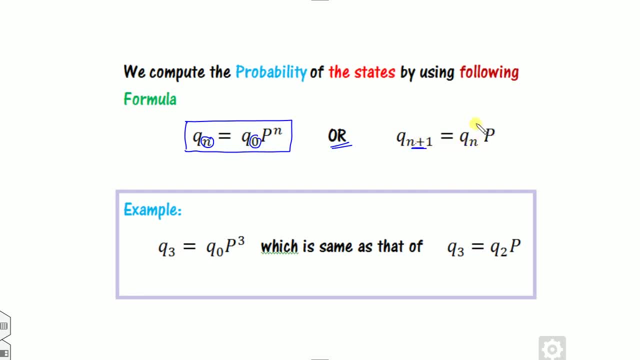 between them is one so had rated as a one. so what is the meaning? is, if i just calculate the value of the ko3, what is the q3 is? that is the probability after the third step or the third day. it means i can either written as: ko3 is equal to ko0, ko0 is my initial probability and the difference 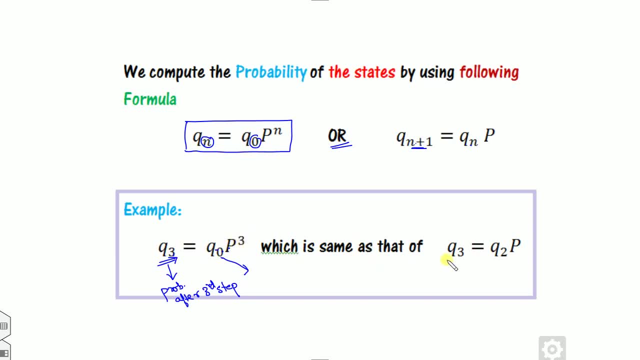 between. the time length is three, so i can write as three, or you can write this way also b, so ko3 is equal to ko2. the difference is: but since ko2 is unknown, so how you find the ko2 is either ko1, difference is one, so you can write one. how to find ko1 is ko0 and p, so if you substitute ko1 here it 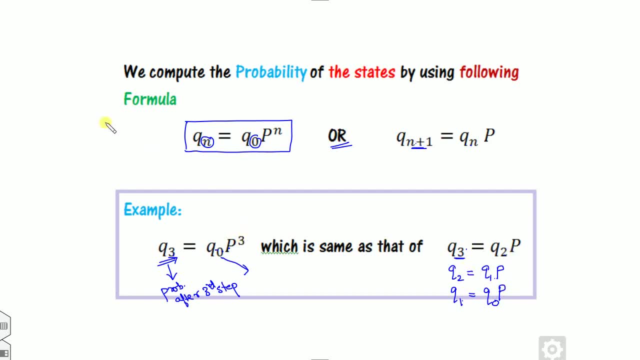 means ko2, p square and then finally reach. here it is important to know that ko0 and the capital p are known to you in every statement. okay, in every statement. these two things are known to you. but how to calculate the p raised power n, this is unknown. p raised power cube is unknown. that we will try to learn in this video, so assume. 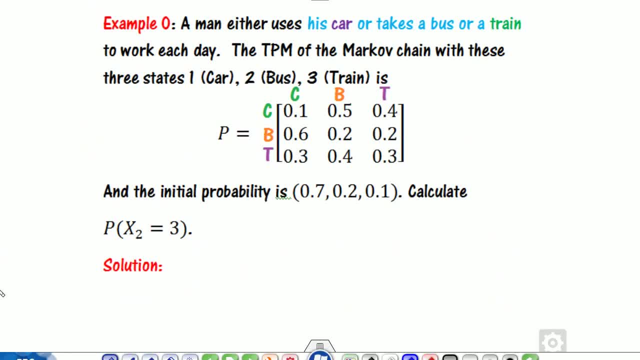 that the first example is how to find the probabilities of such types. a man either use his car or train, or a bus or a train to work each day. the transition probability matrix of these three, because since there are the three states- car, car, bus and the train- and the representation is here- and then the initial probability of choosing. 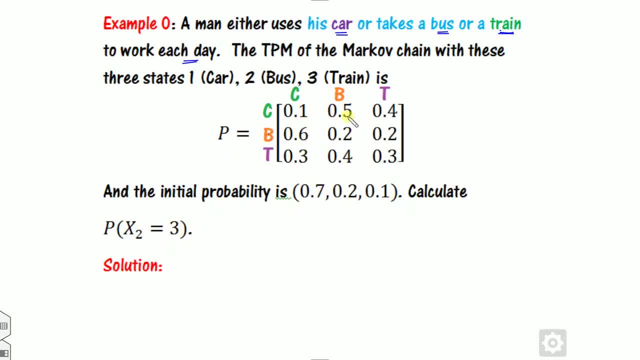 this is so, and so what is the meaning of this? first first thing is that. what is the meaning of this point five? look at that always. remember. this is the past behavior. this is column. represent my future. okay, this is my yesterday, this is my present. what is the meaning of this? if the person 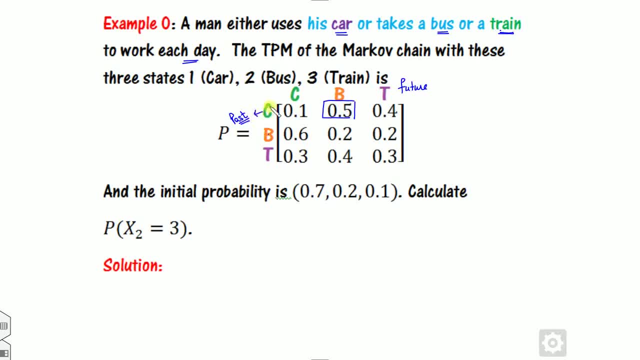 uses the car on the last day to go to the work, then on the next day he uses the bus to go to the work, the chances is 50 percentage. similarly, if i use, if i call as 0.3 means if the person used the train to go to the office in the last day, in the next day he will use again the train. 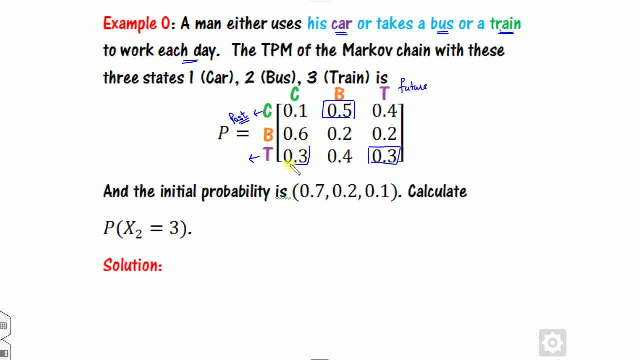 this probability is by 0.3. similarly, like this: if the person used the train in the last day to go to your office, then in the next day he will use the car to go to the office. the chances will be 30 and this initial probabilities and you have to calculate this. 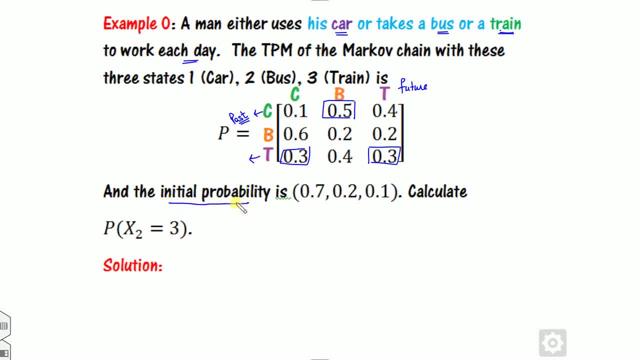 so there are the two things one is called as the initial probability, and what is the physical meaning of it? i just explained them. so what is the physical meaning of this? and since there are the three states, that is, the c, b and t, so this you can't change the order of their states. so here: 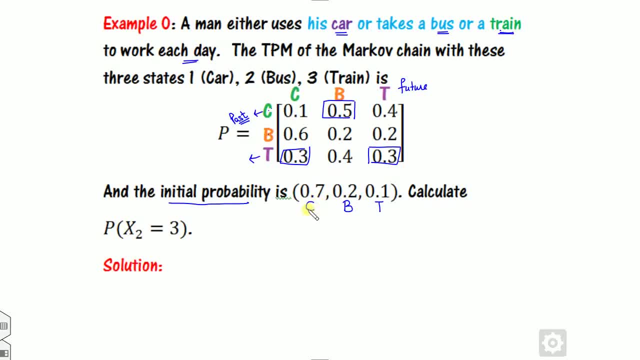 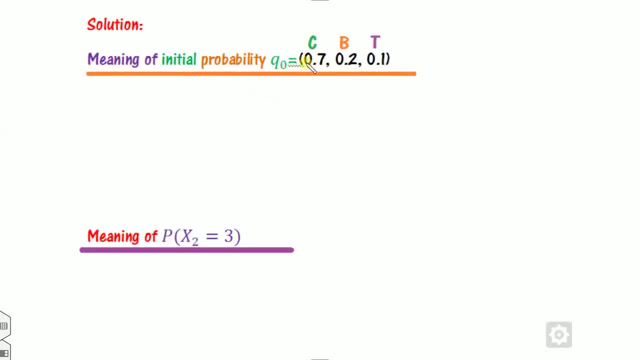 here if represented as a c b t, so you have to write that c, b t instead of the b c t and so on. so what is the physical meaning of this? so 0.7 means that is a 70. so what is the meaning is? 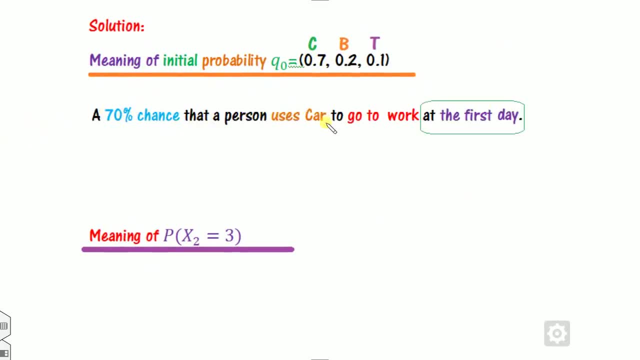 a 70 percent chance is that a person use car to go to the work at the first day. that's why this is called as the initial probability, so either person can use the car or a bus or a train. so what is the chance is, that he can use a car on the first day is 70. similarly for the 20 and the. 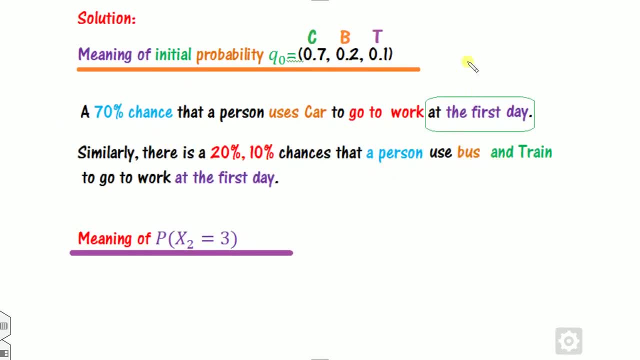 10 for the chances he can use the bus or the train. if in the statement it is given that the person always use the car on the first day to go to the office, then what is the q0 is: always use the car, so the probability is one. others will be zero. we remember that the sum of them will be a one. 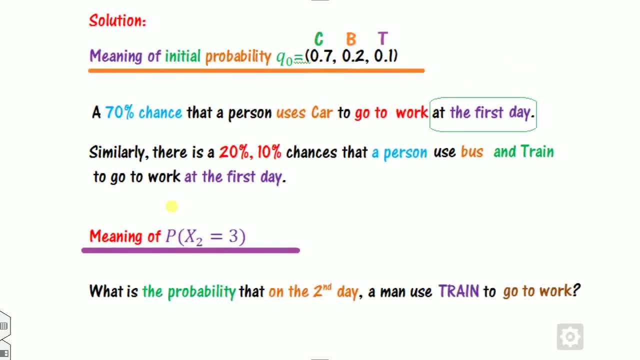 and what is the probability of the car to go to the office? meaning of this is: look at that. this is my state, this is my time. this is my time. this is my state. so what is the three third state? is my train? so in in this, we have to find the probability that. 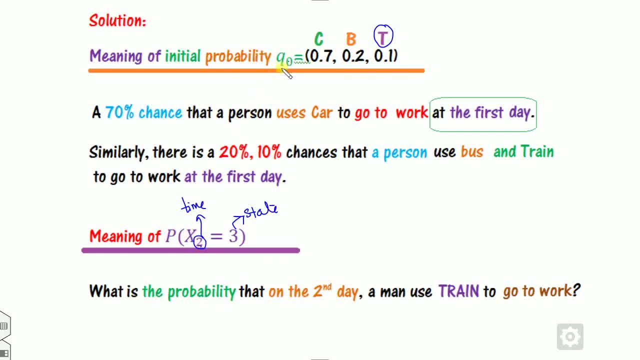 if i call it zero. so what is the difference between them is two. so on the second day a man used train to the work. initially, we know that there is a 10 percent chances that a man used the train to go to office. but what is the probability that on the second day, 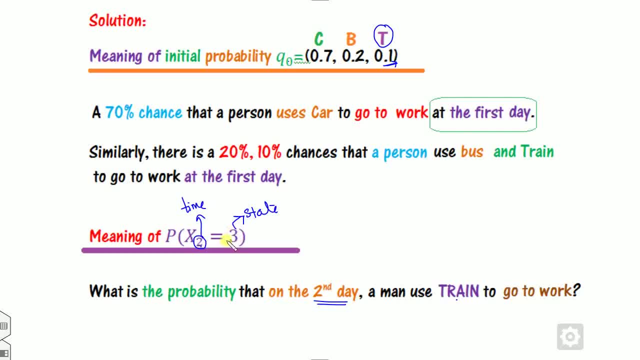 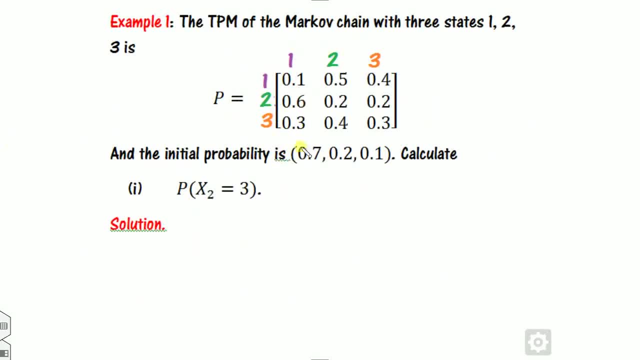 if, what is the probability that on the second day a man uses the train to go to the world? so that's the task of these problems. so how to calculate the problems? are here the same example i have considered. so remember, i have to calculate this. so what is the meaning? is i 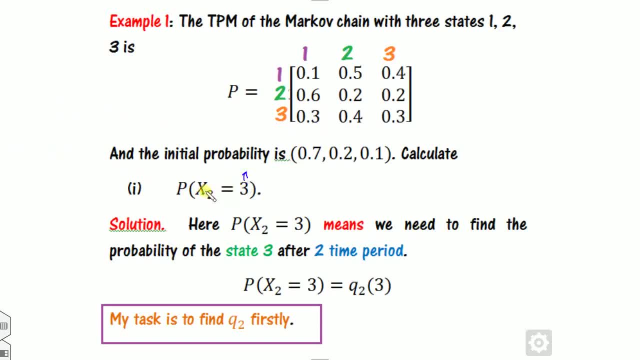 again, probability of the state: three after the time two. so i can represent here as q of this and the state is there, so in. so for this we need to calculate the q2. so the formula for the q2 is: either you can use q1, the difference is time period is one, so you. 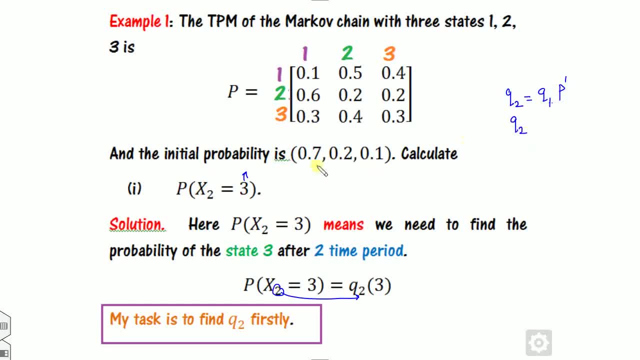 can use as a one or, since it is the initial, is given to you, so initial is q0, so q0. the difference is p2, so you can use either of them. if you use the first one, there is a need to calculate the q1. firstly, since it is not a q1, it is a initial, so q0. so you can use either of them. so. 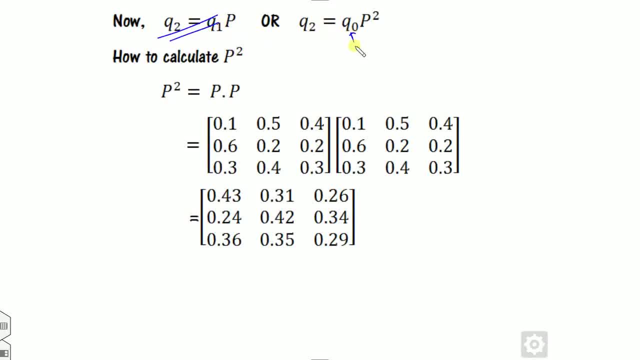 i have to use this one because q0 is given to you. i always prefer use always this formula: qn is q0, p raise power n. okay, so in order to calculate the p scale, because q0 is known to you, only need to calculate the p square. so how you calculate p square is nothing but the p multiply p. 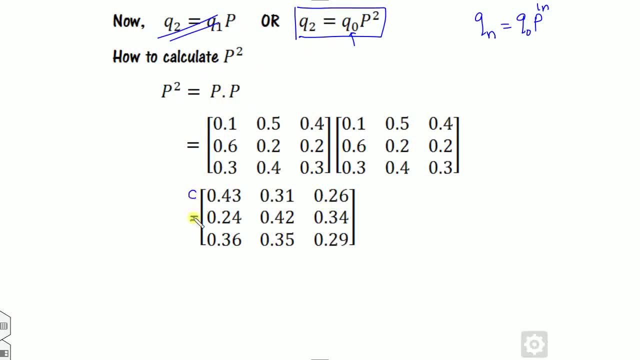 so you simply multiply them, so we will see that in a minute- is that this is the car, this is the bus, this is the train. so so what is the meaning of this? this 0.24 meaning is a person, this is a p square, so it means: after the two days. 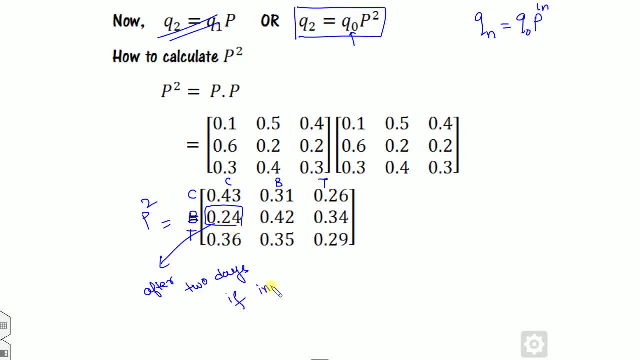 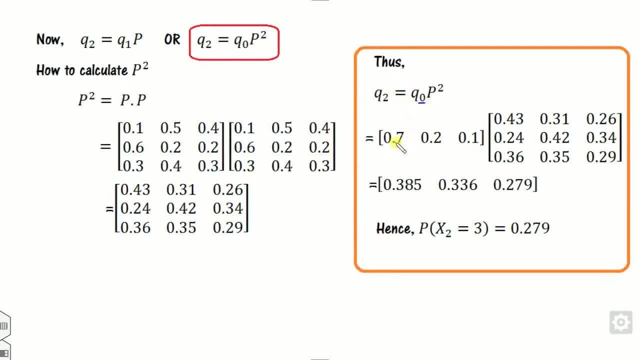 if a person initially used there is a bus, then in the next day he will use the car. the probability will be 24 percent. now substitute this p square value in here. you will get the requirements. so ku0 is given to be 721. multiply this, so this is the probability for the car. this is the probability. 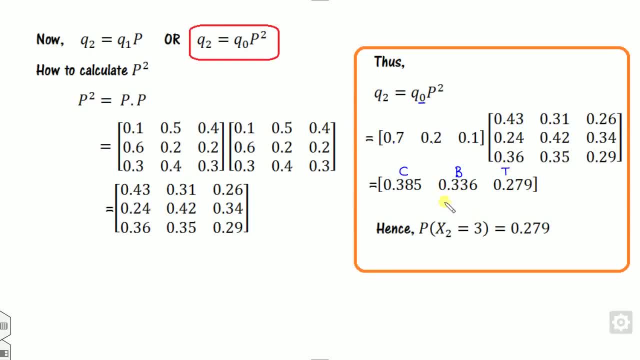 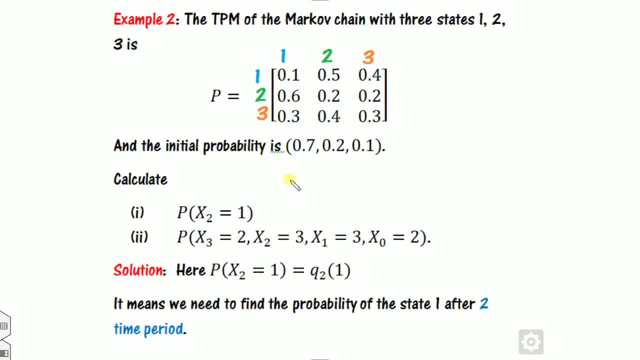 for the bus. this is the probability for the train. okay, so look at that. we are finding the probability of the third stage. that is this. so the answer is 27.9 percent chances that he will use the third state after the two times we at. one more example is there. so here we have discussed the two parts since 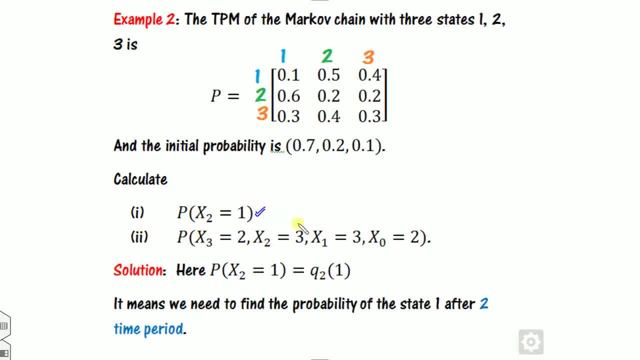 this part. one is only for finding the probability of the state. so right now we are not discussing here. it will discuss in the next lecture. so how you write this is: x2 is equal to 1, means q of 2 after finding q2 and we have to check the position 1. so this is the initial probability. so 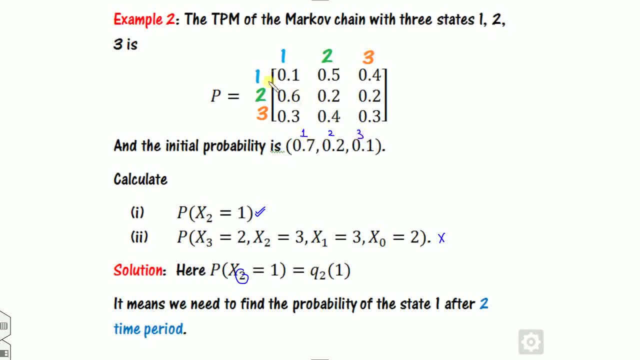 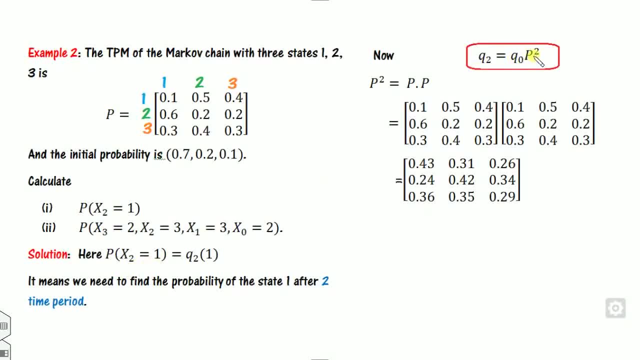 it will be 1, 2 and 3. look at the states are remain there. so how you find? you find the ko2 is so look at that. this. so ko2 is nothing but the ko0 p square. now calculate p square is p multiply p. okay, so this is a state one, this is a state two, three. one, two, three. so 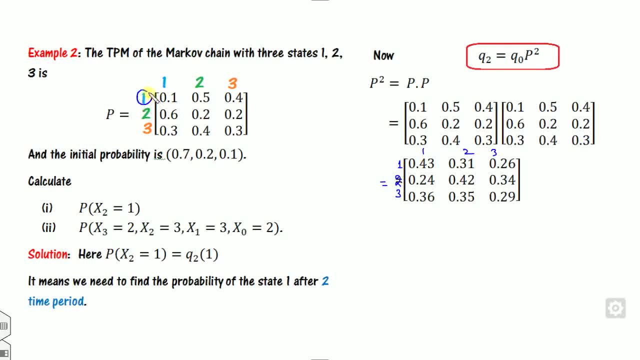 look at that. what is the meaning is if he initially used the state one- if i call this again one- as a car. so if the person used the car in the first day, in the next day he will use the car. the chances will be 10 percentage. on the other hand, after the second day, p2 means second day after the second day. 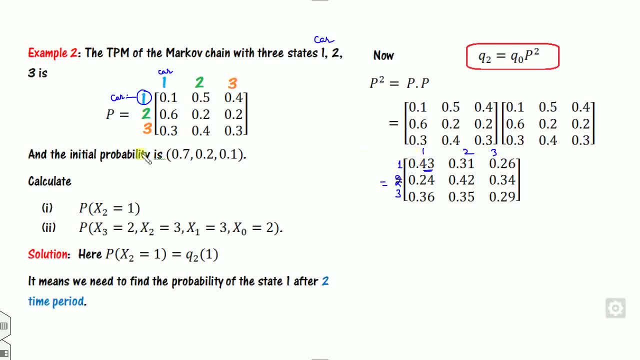 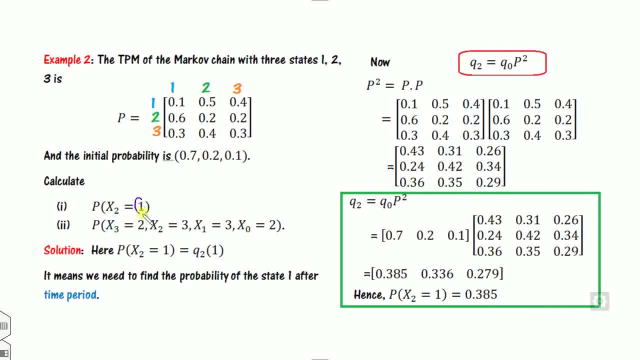 the chances will be 43 percentage if we use the same. now we need to find the ko2. so substitute value, here you will get. now i need to calculate the one. so look at that. one is my first state. so this is my first state. next example: three boys, abc, are throwing a ball. 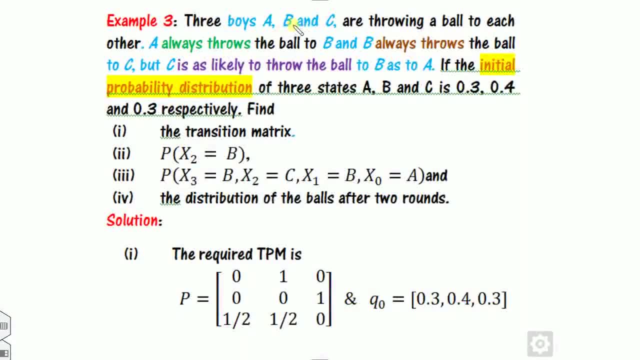 to each others. so it means that there is a three cross, three tpm is there. so you have to find the three cross three. there is a, b and c, a, b and c. so a always throw the ball to the b, so a always throw the ball to the b. so it means this value is one and since the sum will be one in the tpm, 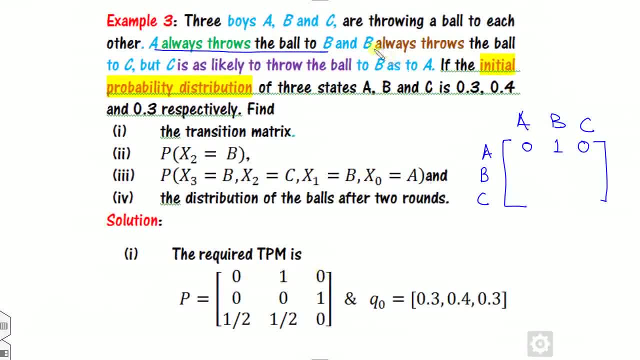 so the rest one will be zero. similarly, b always throw the ball to the c, so b a, b c. so b always throw the ball to the c, so c will be one. other are zero. and, but c is likely to throw the ball to the b. as to the a, it means whatever the c is likely, so a is same as that of the b. 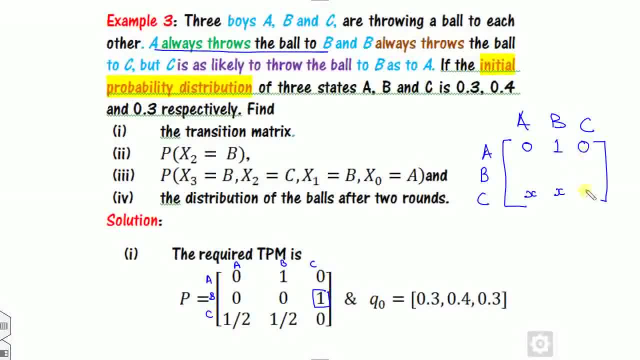 and it is given that c can never throw the b, so the value is zero. so how you find this is: since it is a tpm, so the sum will be one, so you will get x is by half, so the required probability will be here. and what is that? the initial distribution probability. 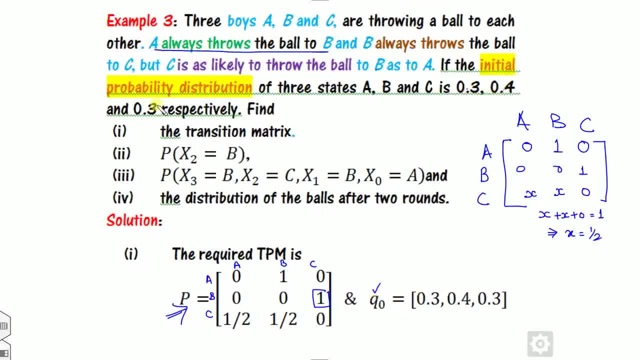 initial means ko0, is given to you three, four and three, so this is the a, this is b and c. look at that. you can't change the scenario of this abc. so construct the tpm. you have already drawn that. calculate this. now this, i can calculate that. look at that. this. so, since it is a chain, so it will be. 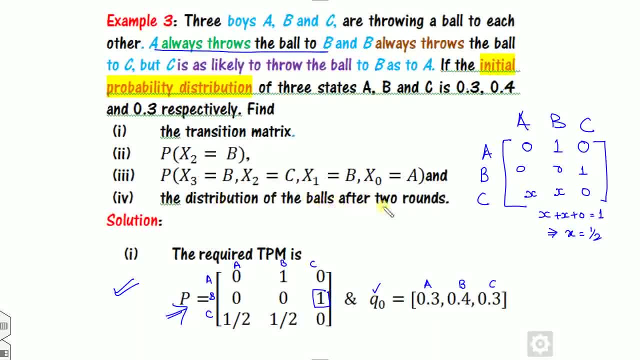 the next lecture: distribution of the balls after the two rounds. so distribution, so that is means you have to calculate this after the two round. it means you need to calculate the q2, because distribution means abc, so that's the state. so you have to calculate q2 for this part, while in this part how you calculate. 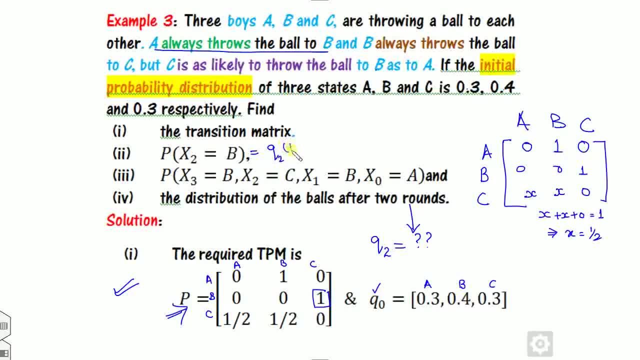 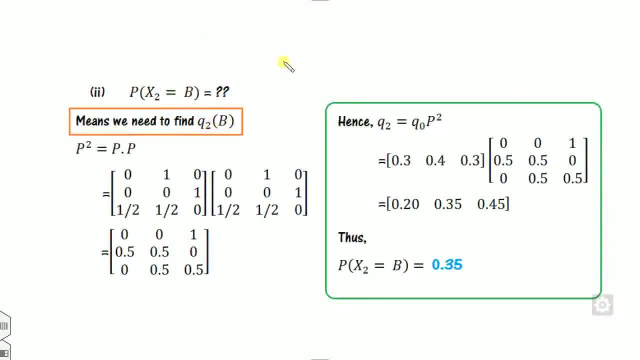 that you have to calculate q2 and find their values. b. b means that is the second position, so that's very simple. is that you need to calculate this? so what is the q2 is zero p square. so you calculate the p square. this is a p square, now substitute here. so this is the part. 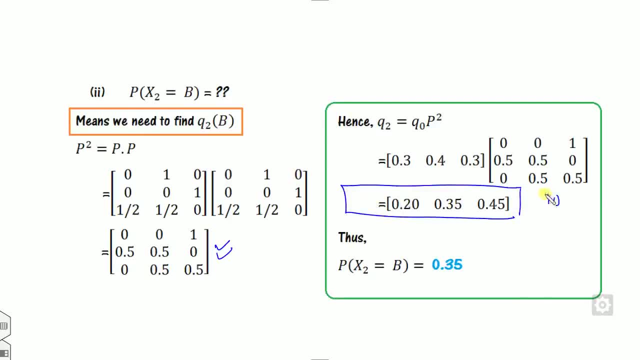 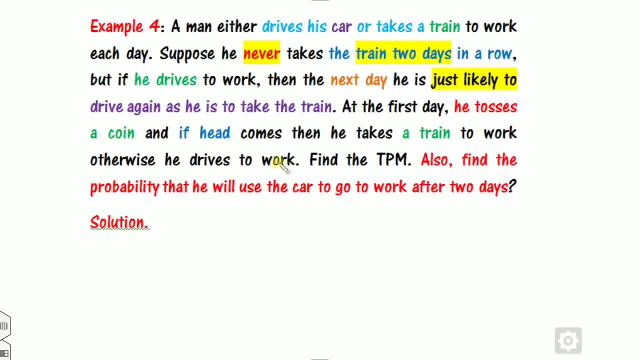 of their fourth answer and among this you need only to calculate the b. here is my a, this is b, this is c. so this is my b and this is the market share. this is the share of their distribution of the bonus. so, last example, is there a man either drive his car train or drive his car to the market? 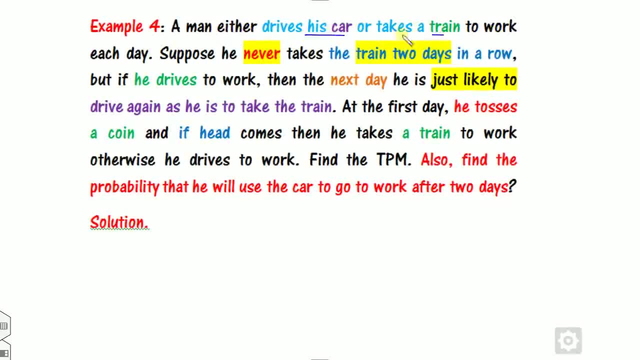 or take a train to work. so there are the two: car and train. so it means there is a two by two matrix that is either a car or train, car or train. suppose he never takes that train two days in a row, but he likely to drive and so on. so you can read this pause video and read that. so what is? 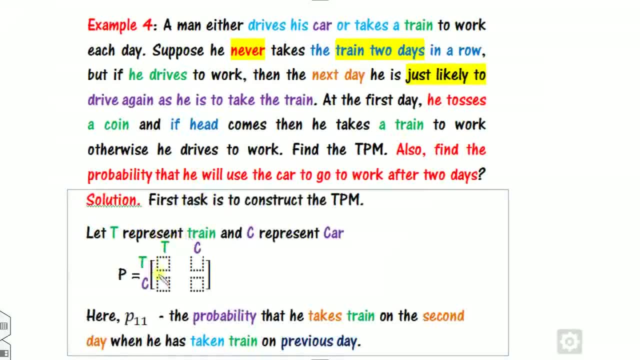 that. so there is a two. i call as three represent train and car are there. so what is the meaning of this? it means that is a probability. first value is the probability that a person will drive a car. if a person takes a train in the last day, again in the next day he will take the train, but it is. 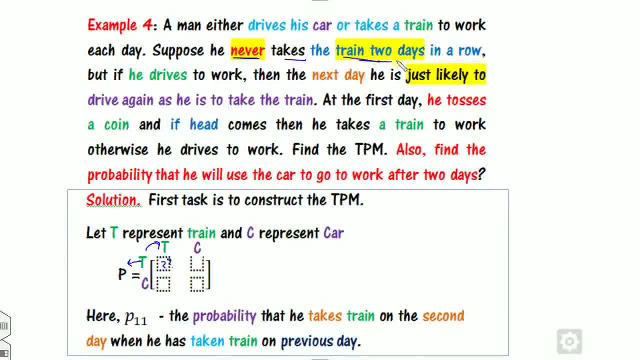 given that he never takes the train two days in a row, it means if he previously used the train, the next day he will never use the train. so the answer here is zero. okay, train and train will be zero according to this line, and since the sum will be one, so it will definitely be one. what about the? 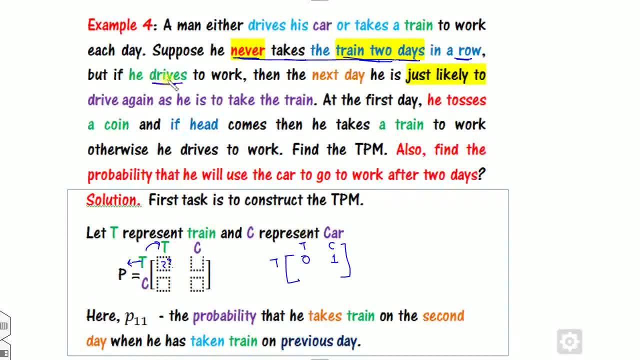 car condition is: if he drives, drives car the next day, then the next day he is just likely to drive again as he like to, between if he likely to be there. so it means that will be. so you can easily find the value of X will be half. so look at that. so why? 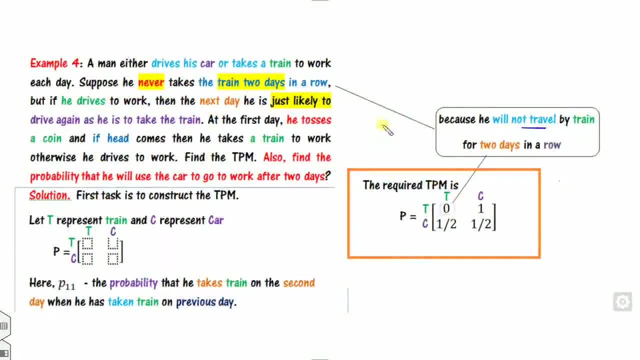 it is 0 because it is given that he is not trained okay. so what is the initial probability? now, what you have to find? that at the first day he tosses a coin. so at the first thing, toss a coin. if head comes he will use the train. so what is the at the initial? 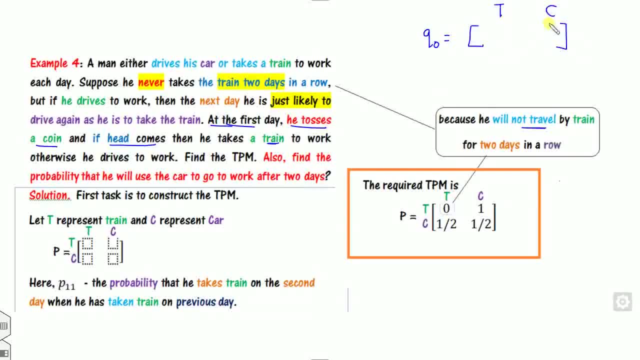 so there are the train and the car. if head comes, he takes the train. so what is the probability of coming? the head, that is the half okay. and what about the remaining? is there is a tail, and since some will be once, it will be okay. so if 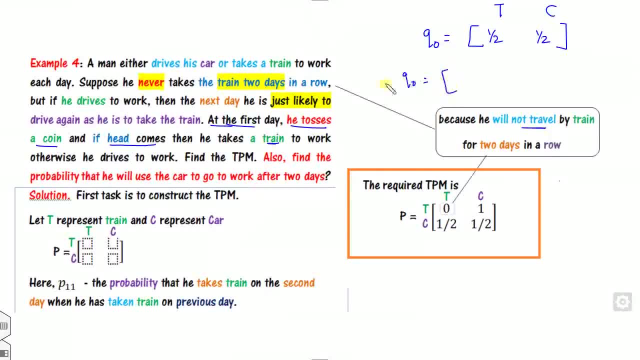 in this example, if I say: consider that there are the same train, car and bus, so in this same case, if head appears, that train will be taken, if tail appears, the bus will taken. so what is the probability of? the tail is half, then it will be zero. okay, so this is the case for the other case. so right now, here is 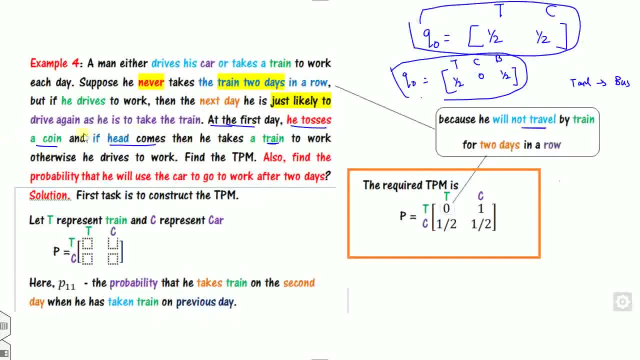 the initial case study. so what is now what will happen is you will get the initial case study. so what is now what will happen is you have to find the TPM that is over, find the probability that he will use the car to go to the work after two days. so it means you have to find the probability. 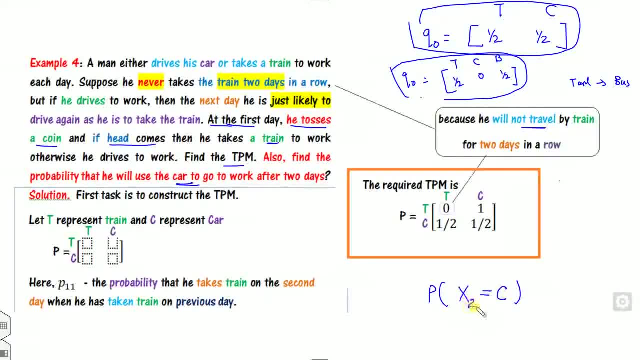 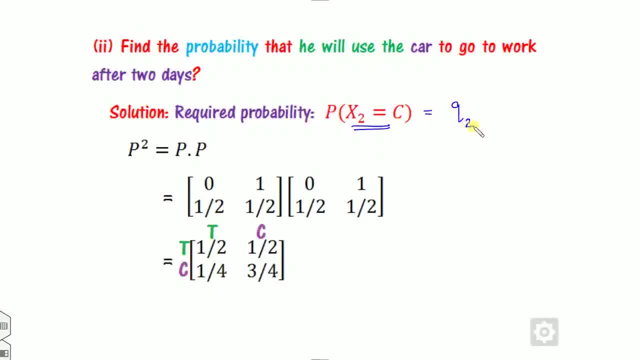 of the car. how many days are there? two days, so that is the minimum. so you have to find this. so how you represent this, as you have to find the ko2 second time and look at the value of the C. so ko2 means you have to find what is the ko2. 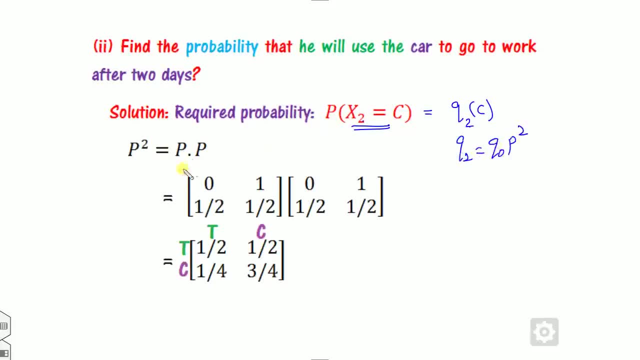 is ko0 p square, so you have to find the value of the C. so you have to find the value of the C, so you have to find the p square. remember that I have used a t firstly and then see later on, so that T and C are here. so now, what is that? 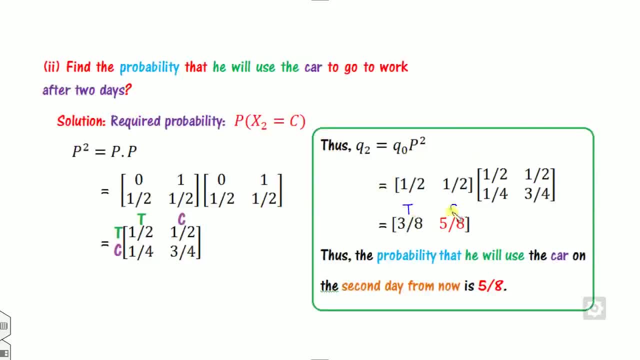 q2 is this is there? a first C is here. so what is there? this is the value of the q2 and you need to find the value of the C. so this will be fiber. so this is the probability that he will use the car on the second day. so I hope you can enjoy. 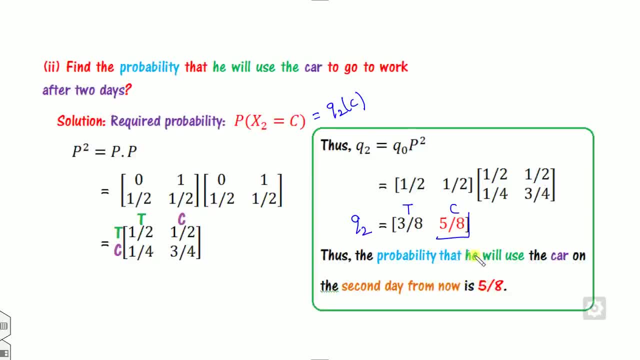 this session be practice mode. listen this, for example: again, i can assure you again that nobody can defeat you in this mark of chain problem. wait for the next video in which we will try to learn the second type of the problem. till then, best of.